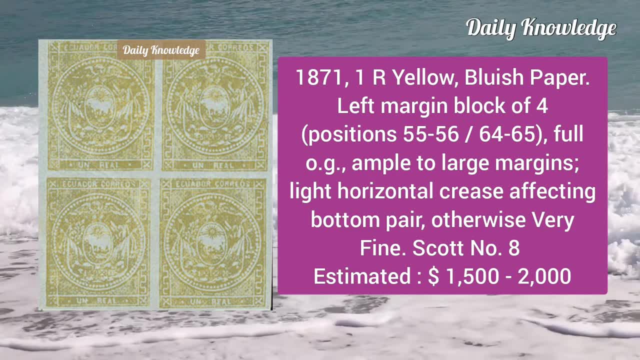 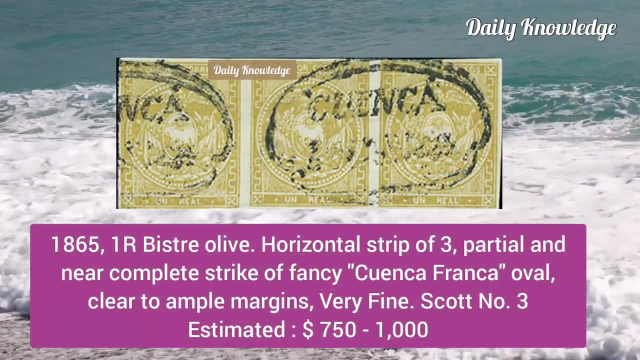 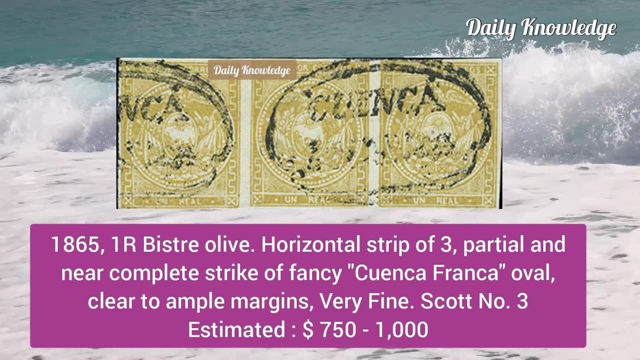 to large margins, Light horizontal grease affecting the bottom bare. otherwise it is very fine. now this is 1865. one hour, mr olive. horizontal strip of three partial and near complete strike of fancy. guenza franca oval dead stamp. it is clear to ample margins and is very fine. 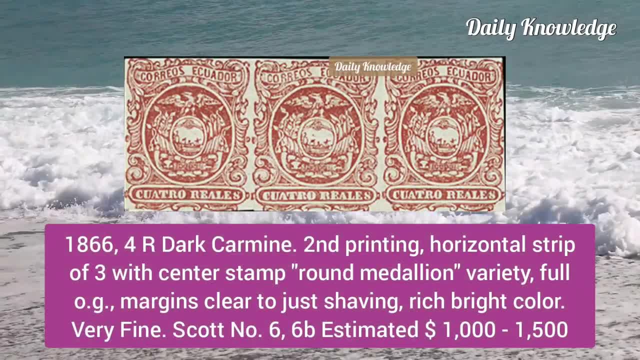 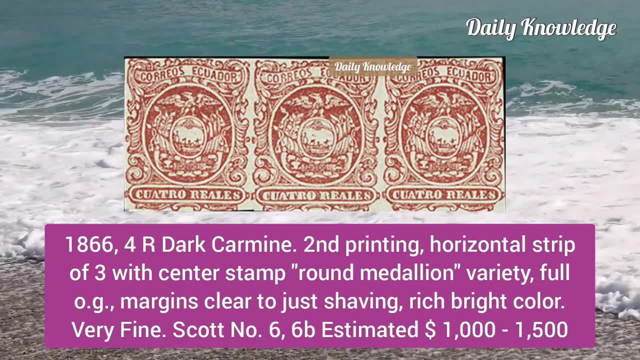 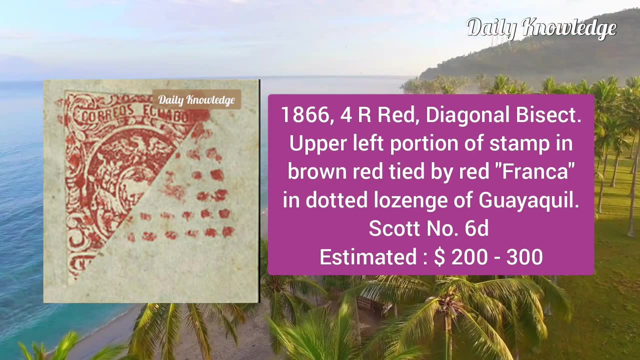 then 1866: four hour jar carmine second printing horizontal strip of three with center stamp, round medallion variety. it has full original gum and margins are clear to just shaving now. next is 1866. four hour red color diagonal bicep, upper left portion of the stamp in brown red tied by 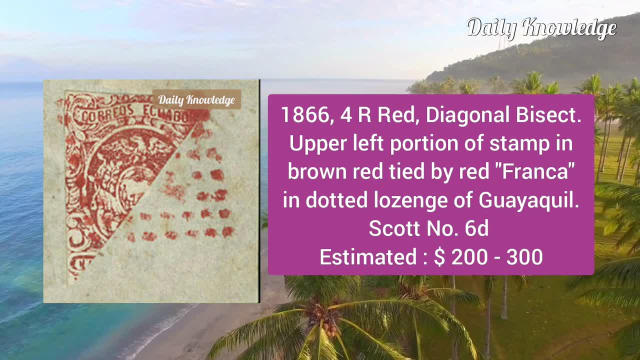 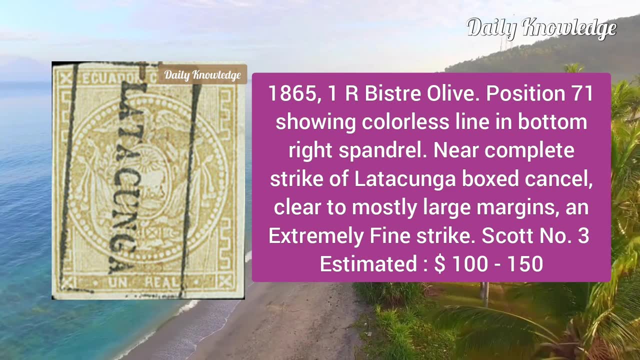 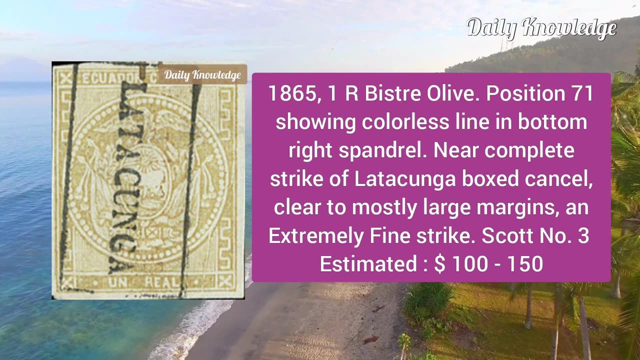 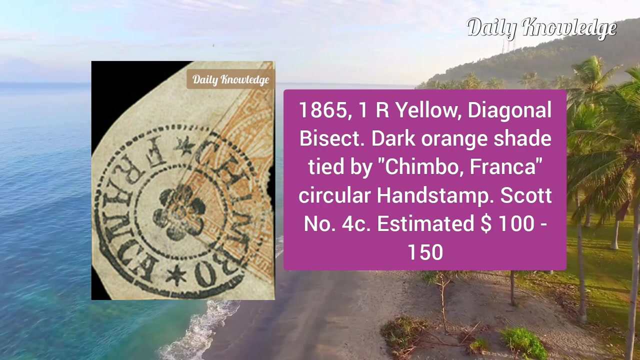 red franca in dotted lozenge of the coin quail in 1865, one hour. mr olive. position 71 showing colorless line in bottom right spent roll near complete strike of laryngea box. to cancel now this stamp is 1865, one hour, yellow color, diagonal bicep. 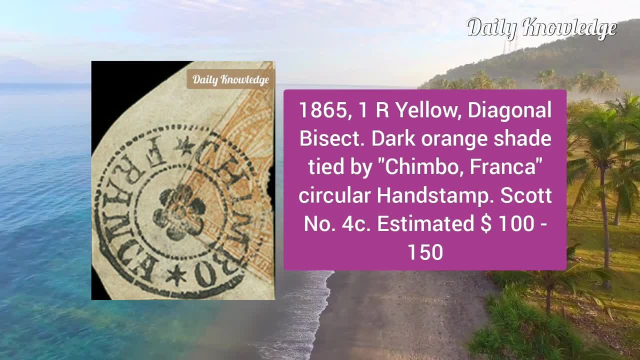 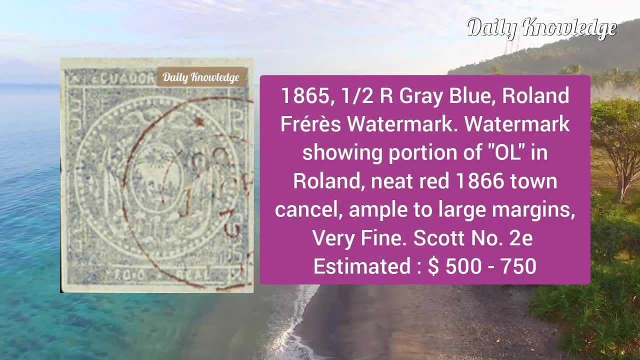 dark orange shade dyed by jumbo franca circular hand stamp and the court number is four c. now this is 1865, half hour. grey blue: roland ferrari's watermark. the watermark showing portion of oval in the center of the lamp color cannot be shown because of theutericồnng. 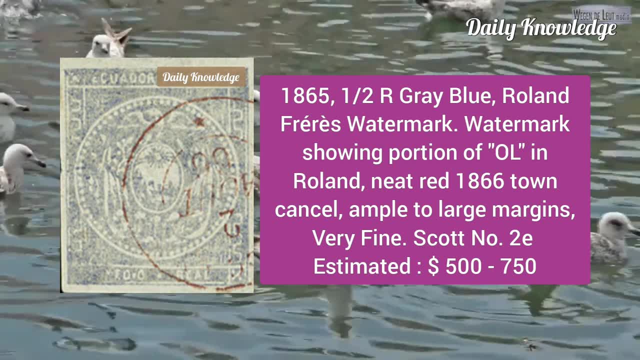 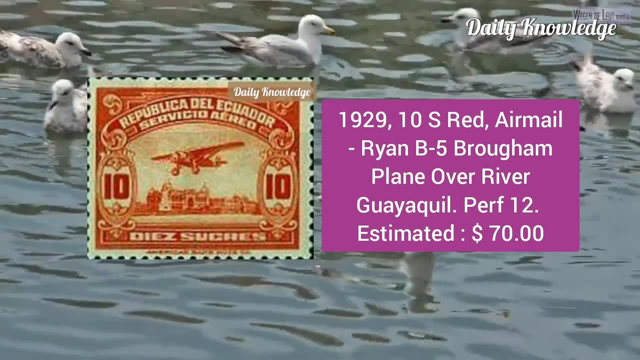 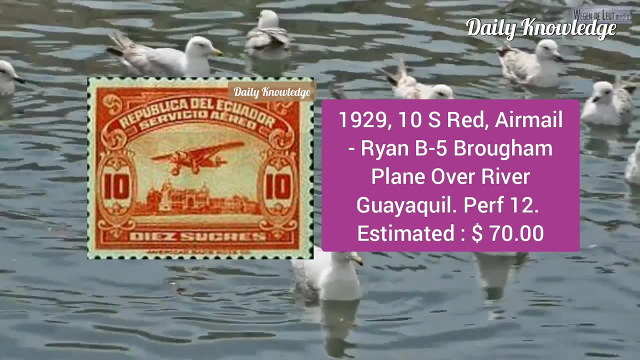 roll it neat: red 1866 town cancer. it is ample to large margins and is very fine. now next step is year 1929, 10 s red color. it is an airmail stamp and it is ryan b5 borkham plane over the river. 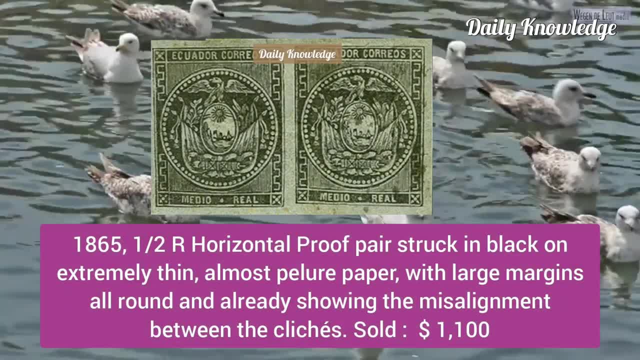 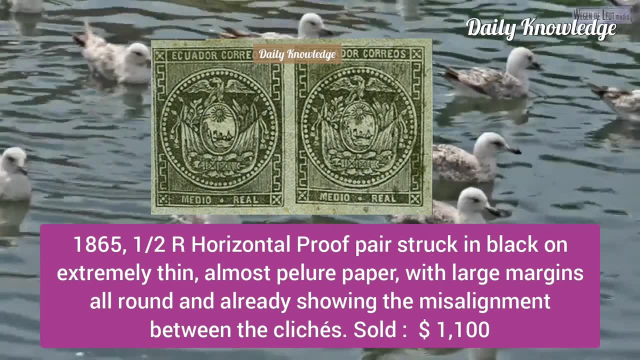 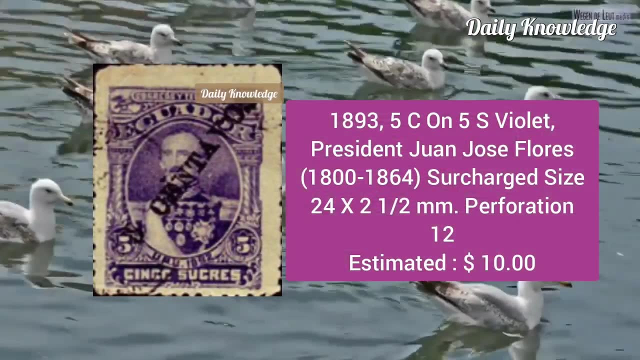 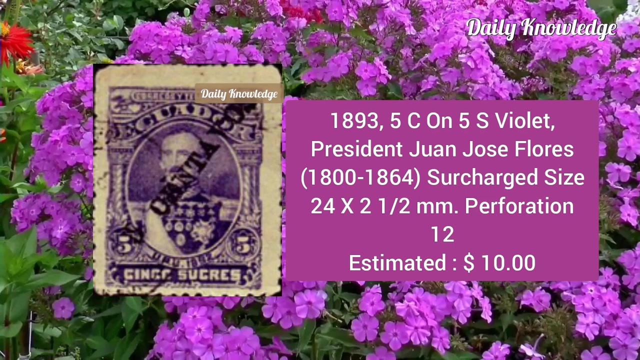 perforation is 12.. 1865, half are horizontal proof pair struck in black on extremely thin, almost pallor paper with large margins all around and already showing the misalignment between the glitches. now, 1893, 5c on 5s, violet president john joe's flores surcharged size 24 times. 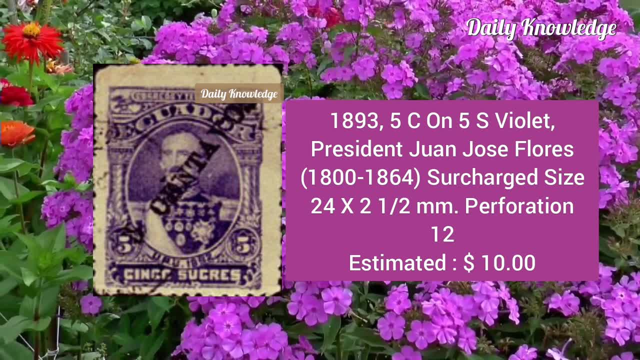 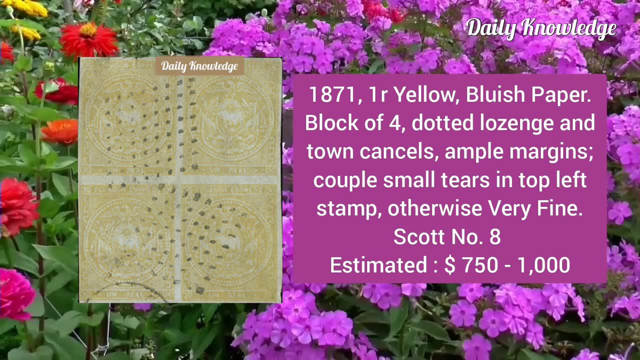 two and a half millimeter perforation is 12.. now 1871 1r yellow bluish paper block of four dotted lozenge and down cancel ample margins. it is a couple small tears in the top left stamp. otherwise it is very fine. 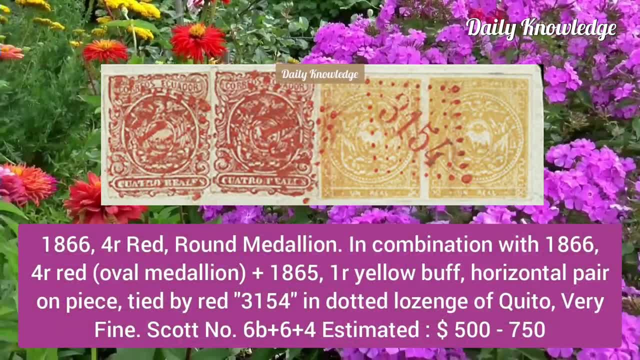 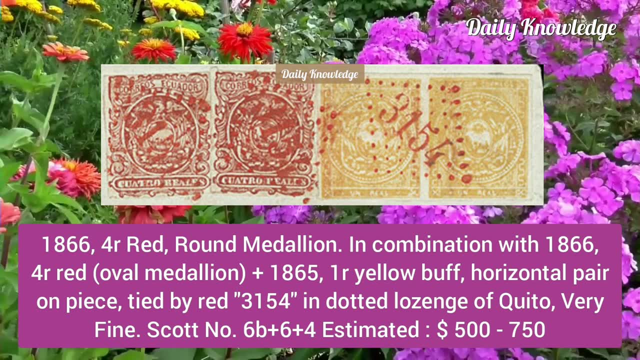 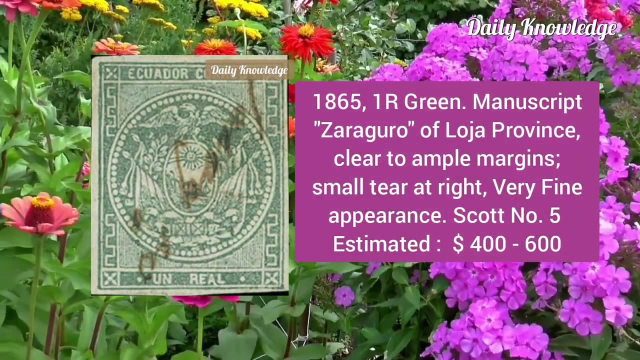 now. next is 1866 4r red round medallion in combination with 1866 4r red oval medallion plus 1865 1r yellow buff horizontal pair on piece. now this is 1865 1r green manuscript of zaragura. 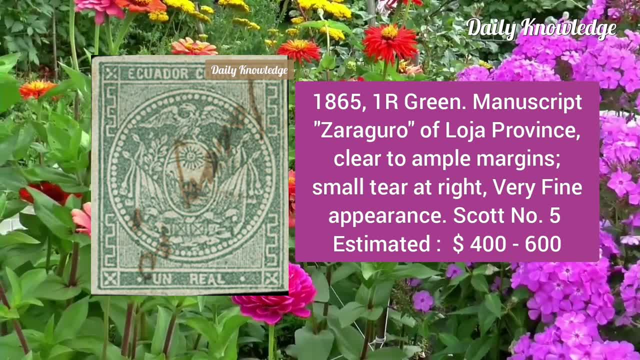 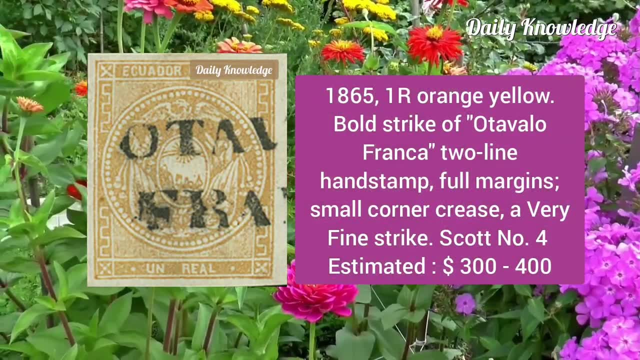 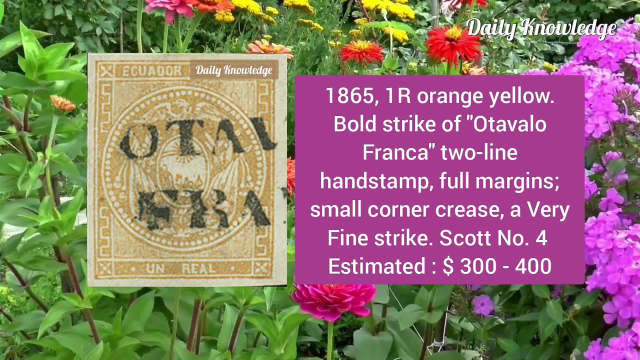 Hansen with red accent libraries, five red感覺 still hurting her. 1865 block of three. one r orange, yellow, but a lot called ojavelo franka do line hand stem. it is full. marching small corner could cause, otherwise it is very fine. 1865 text in the inscription: 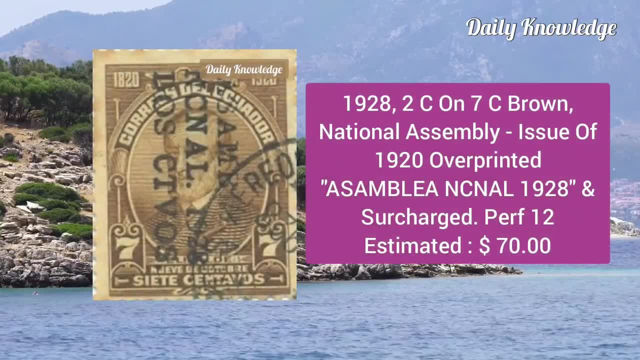 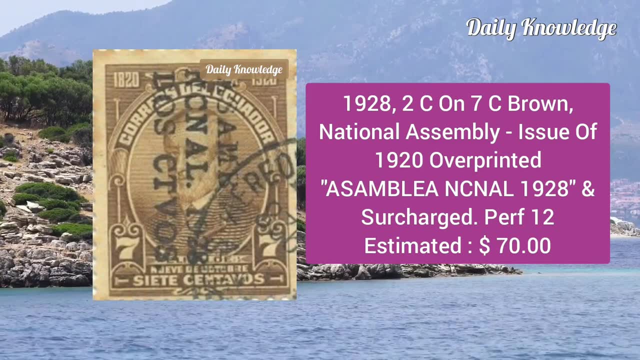 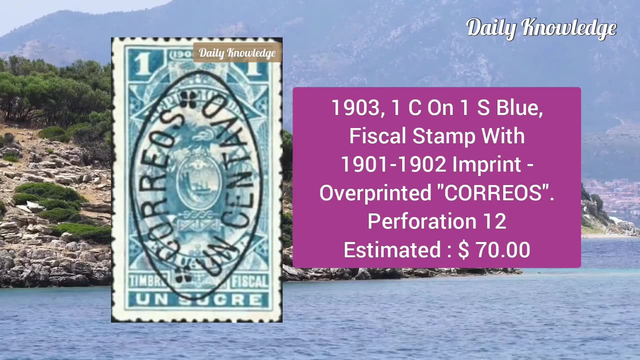 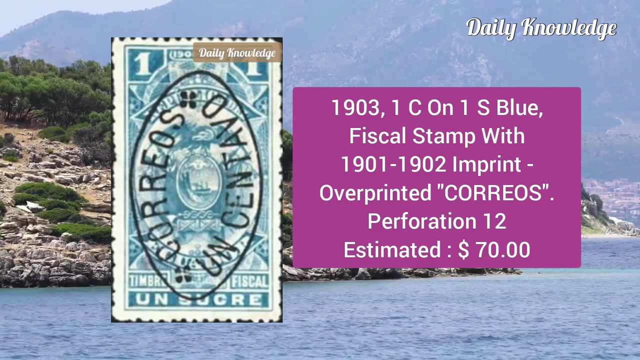 next tip is 1928, two sea on seven sea brown color national assembly issue of 1920, overprinted and surcharged. perforation is 12.. now, 1903, 1c on 1s blue color fiscal stamp with 1901 to 1902 imprint overprint coreos perforation 12.. 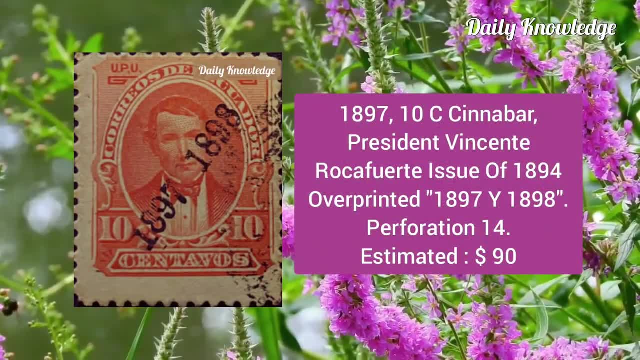 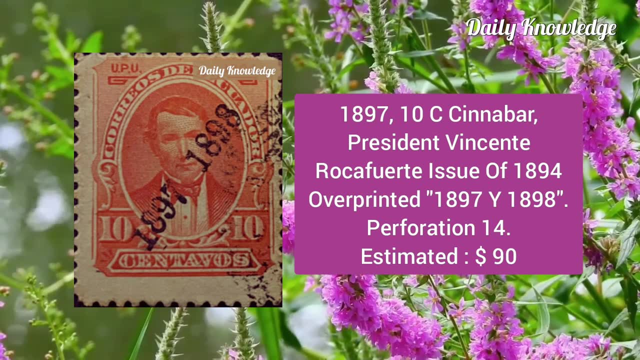 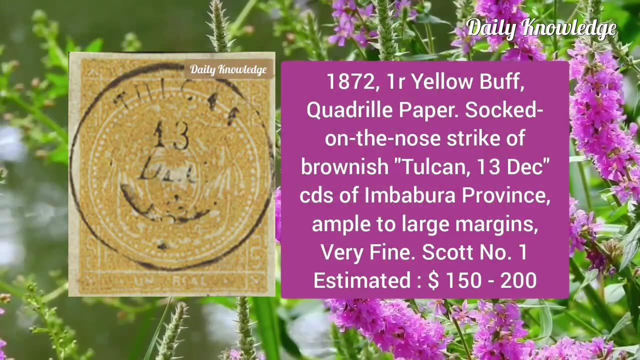 now this is 1897 10c cinnabar president vincenti rocafort, issue of 1894, overprinted 1897 y 1898. now it is perforation 40.. now this is 1872 1r yellow buff cotrail paper. 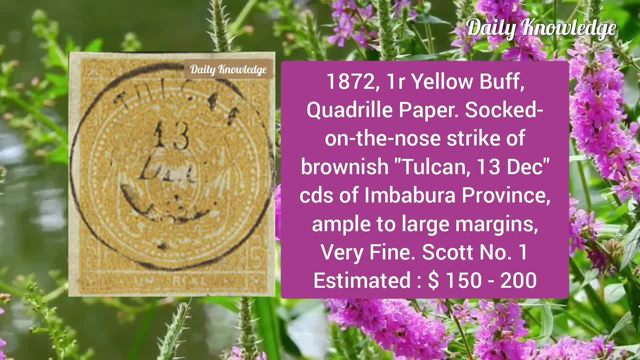 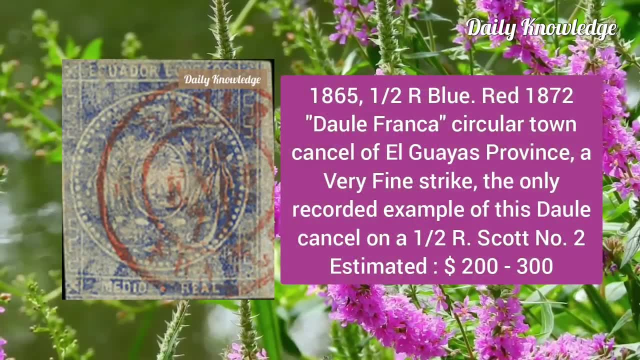 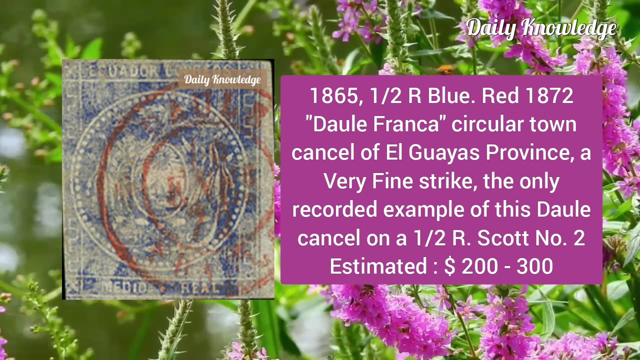 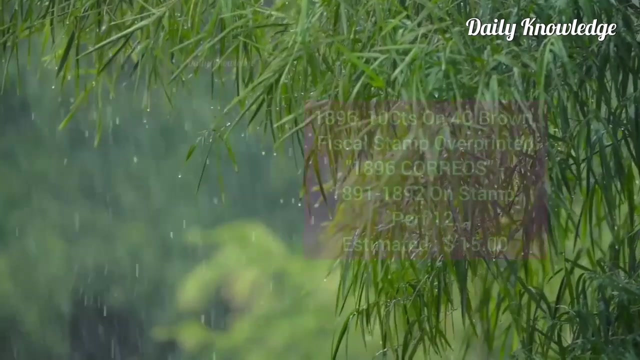 soaked on the nose. strike of brownish tulcan, 13 december. cds of impabura province. it has ample to large margin and is very fine now. 1865, half r blue, color red, 1872, 12 franca circular town cancer of the el guas province. it is a very fine strike and the only recorded example of this dual cancer. 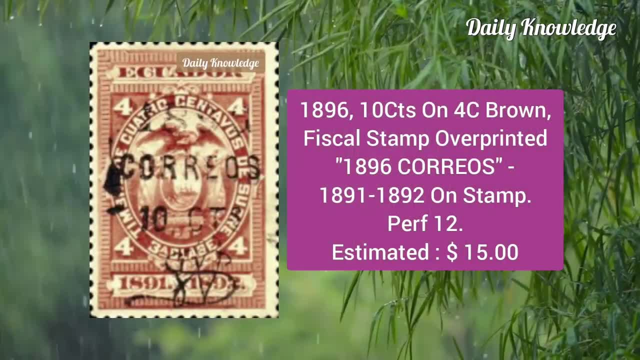 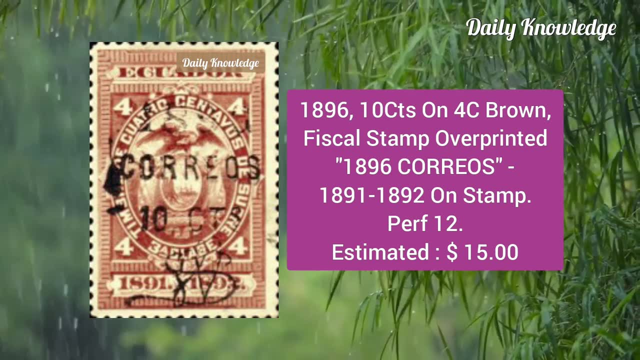 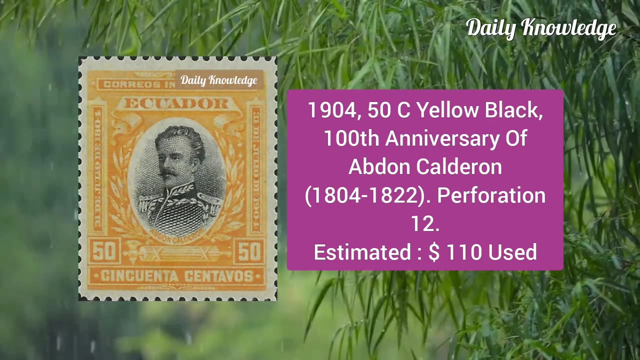 now 1896, 10 cds on 4c brown fiscal stamp over printed 1896 coreos 1891 to 92 on this time and perforation is 12.. now this is 1904, 50c yellow, black color. 100th anniversary of epton calderon. 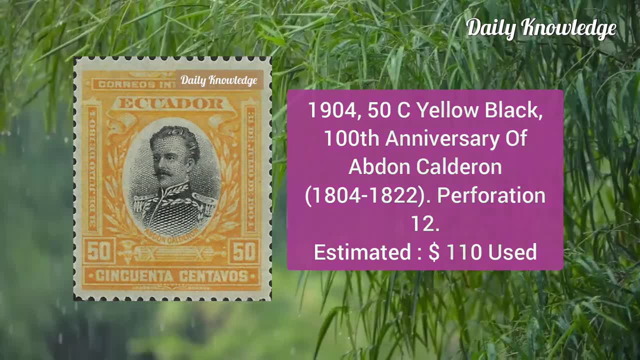 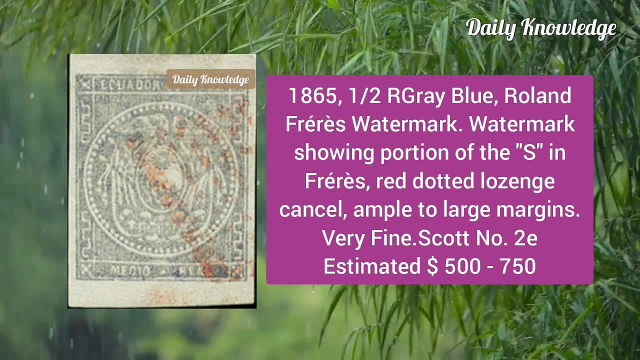 now perforation is 12 and the estimated value is 110 us dollar. now, 1865, half or gray blue roll and fr proportional watermark, the watermark showing person of the s in the frerries, red dotted lozenge cancer. now next is 1865, half, r calderon. perforation is 12 and the estimated value is 110 us dollars. now italian triple dot cancer of novel вниз は. now next is 1867. half are gray blue roll and ladies watermark, the watermark showing portion of the s indie ferris, red dotted lozenge cancer. now next is example of the euphratesruan use of d screws. sign of d freres, red dotted lozenge, ancillary cancer, and next is automobile cancer, cancer now. next is 1865, half r blue cross and 되어 neutral lancet came. next is 1865, half r grey, blue, rauleyn frerries watermark, the watermark. 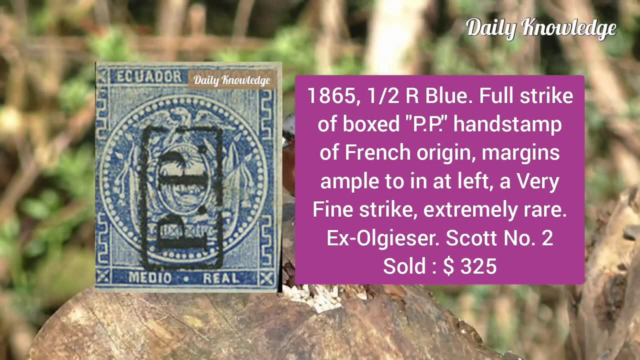 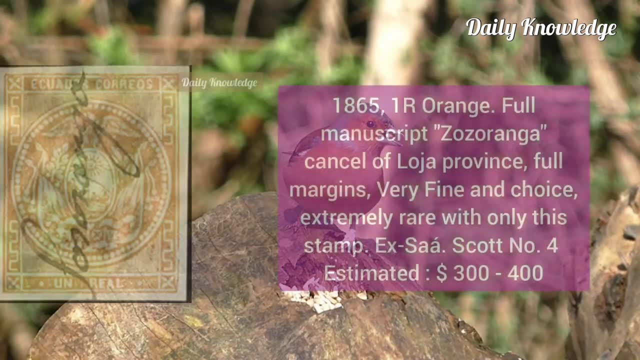 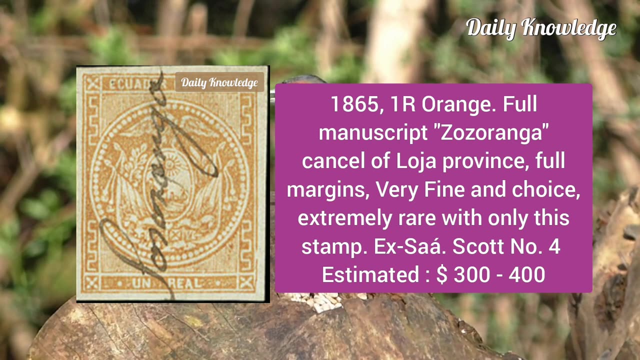 1865, half hour, blue, full strike of boxed pp hand stamp of the french origin. margins are ample to inlet left a very fine strike. now, this is from year 1865, one hour, orange color, full manuscript, zozoranga cancel of the loja province. it has full margin and is very fine. 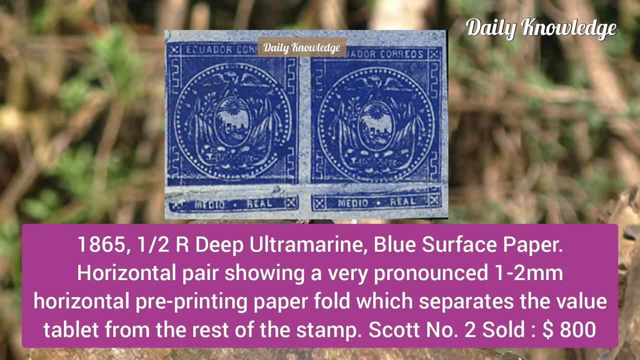 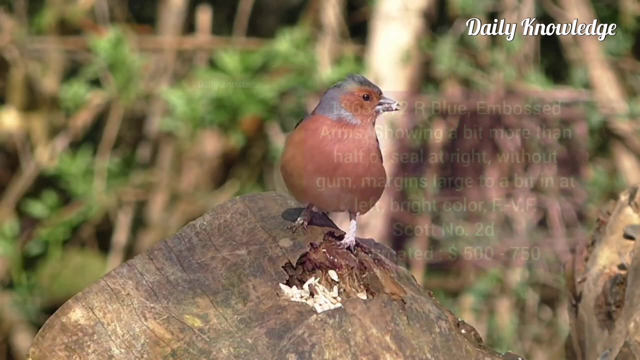 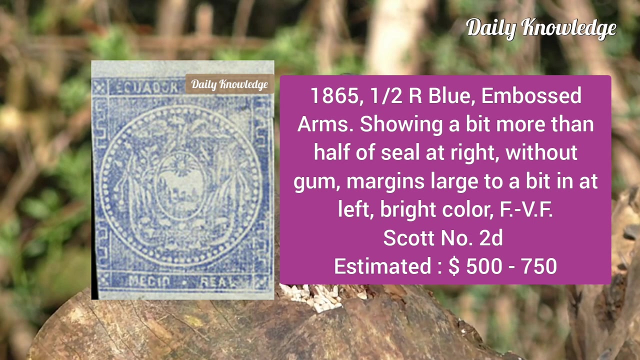 now next is 1865: half hour deep ultramarine blue surface paper horizontal pair showing a very pronounced one to two millimeter horizontal pre-printing paper fold. now next is 1865: half hour blue embossed arm showing a bit more than half of seal at the right. 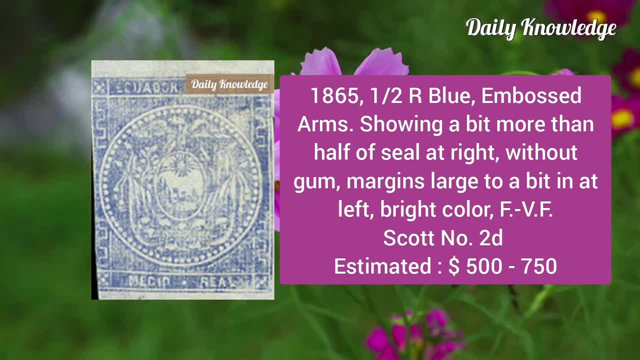 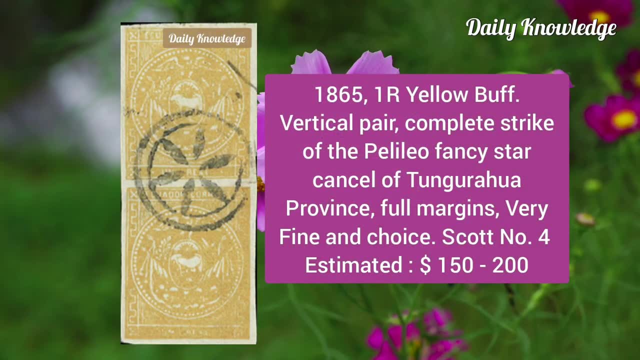 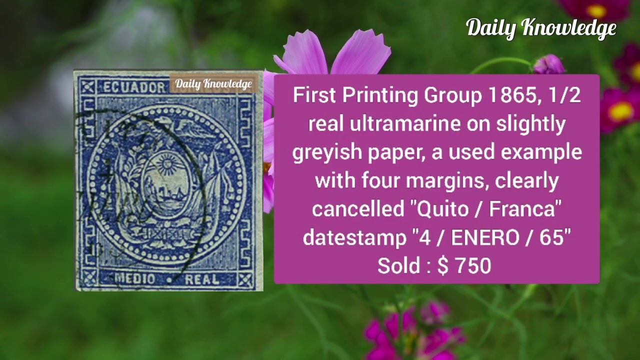 without gum margins, large to a bit in at the left. it is bright color and is fine to verify now. this is 1865: one hour yellow puff vertical pair. complete strike of the belly low fancy star cancel of the tangurahua promise. it has full margin and is very fine now. this is first printing. 1865: half hour ultramarine on slightly. 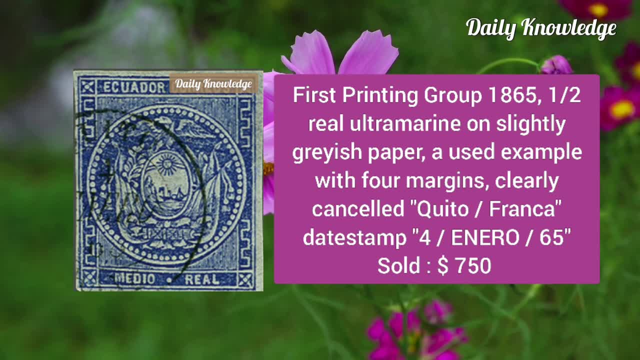 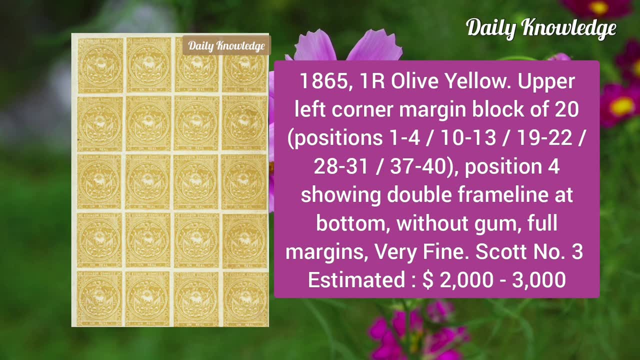 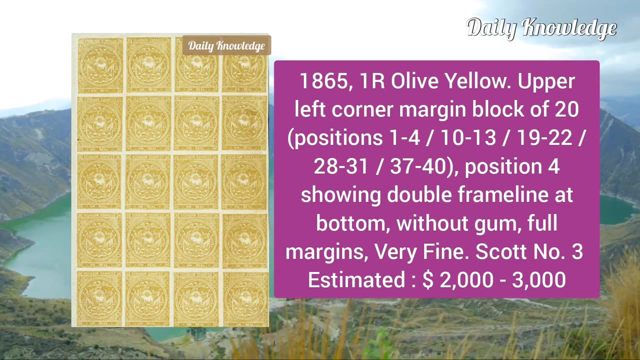 grayish paper, a used example with four margins and clearly canceled. guido franca did stem. now next is 1865: one hour. olive, yellow upper left corner margin block of 20, position 4, showing double frame line at the bottom which is without gum and has full margins and is very fine. 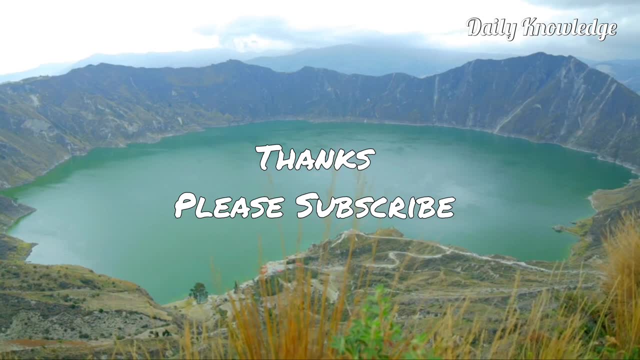 okay, friends, thanks for watching. please like share, comment and subscribe to my youtube channel for more informative videos.